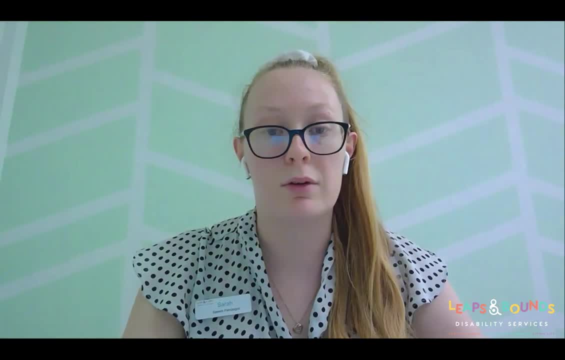 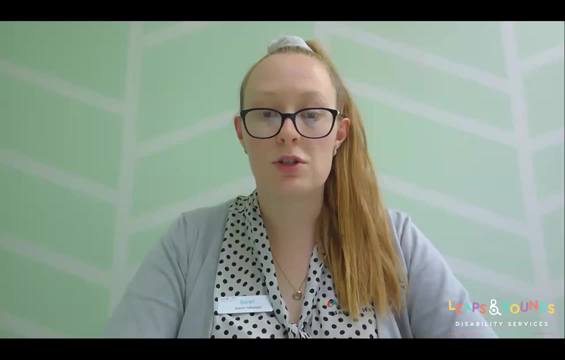 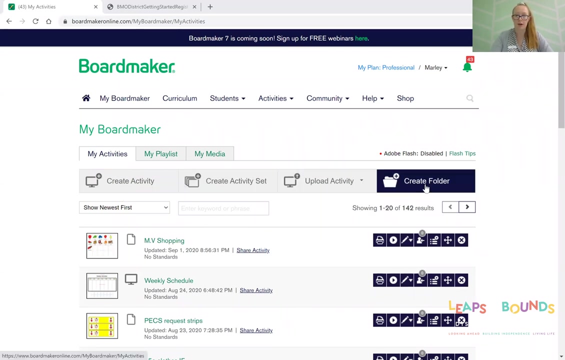 you guys could maybe use it within the home to make your own visual aids. So I'll just quickly pull up my page and we can get started. So first you want to go ahead and log into Boardmaker. So your page should look like this: We have a bunch of stuff on the toolbar. 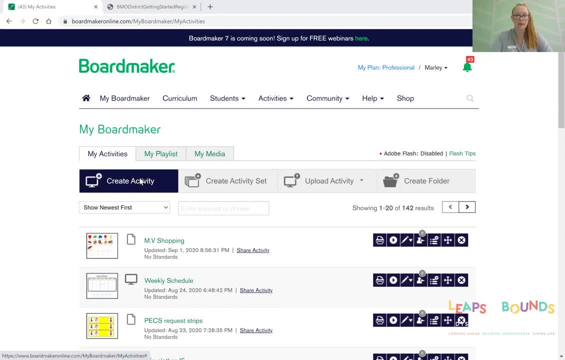 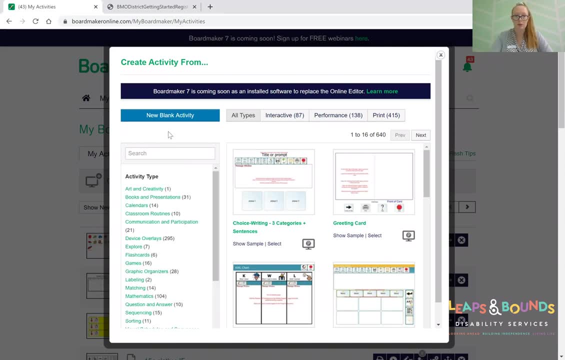 here So we can select. however, I'm going to go create activity. It has a range of different templates that you can search for and look for, to give you ideas and maybe build off. However, we're just going to go ahead and do a new blank activity today. Okay, so we've. 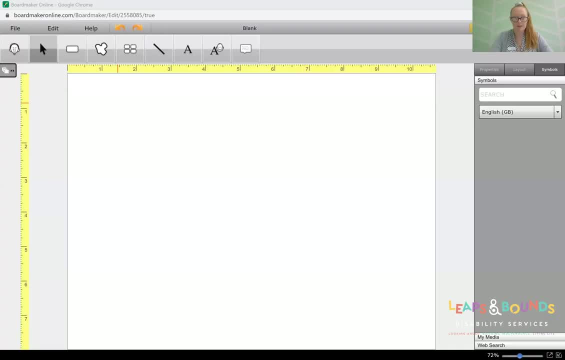 opened up our new blank activity. It should look a little like this. You can see we've got a toolbar up here. So we've got the Boardmaker Man selection tool that helps us click and drag. We've got our Cellmaker, a free form kind of button in Cellmaker. 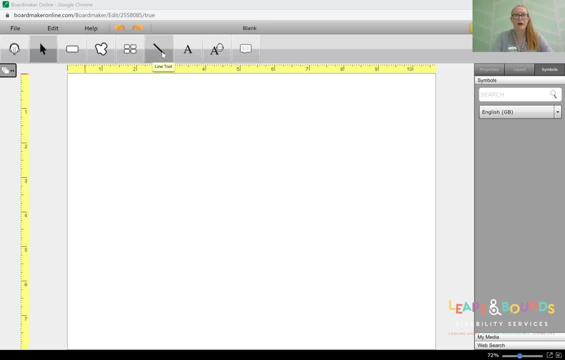 Our Spray tool which helps us copy all the cells, a line tool, a labeling tool and so on. So we'll go ahead and make our first cell. So we'll go ahead and click on the cell button and then it should appear like this and we can drag out, We can use our measurements. 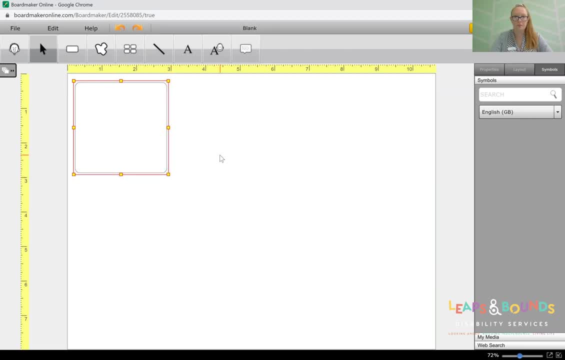 on the side to help us kind of make our cell size. So there's our first cell. We can then use the Spray tool and then drag our cells. So then we've got the same size cells, but there's just more of them. We're going to go ahead and then add in a symbol, So you 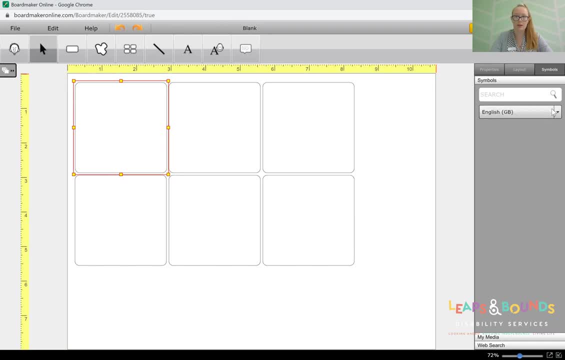 can see here. if you click on the cell, it'll come up with this side kind of toolbar. We can then search for, say, a car, Pressing enter, And then I'm going to pick this car here. So I'm going to go ahead and click on it and drag it over to the cell and then release. 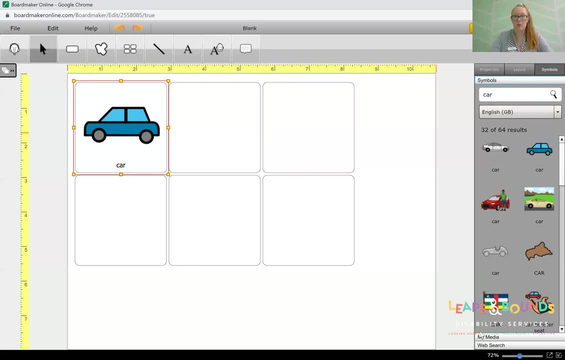 So then we've got our car in the cell. there We can also search for cars in our media or saved, or we can search the web for a car picture that we might like to make it more relatable. So if we're looking for a specific car like a Lamborghini or a Maserati, we can